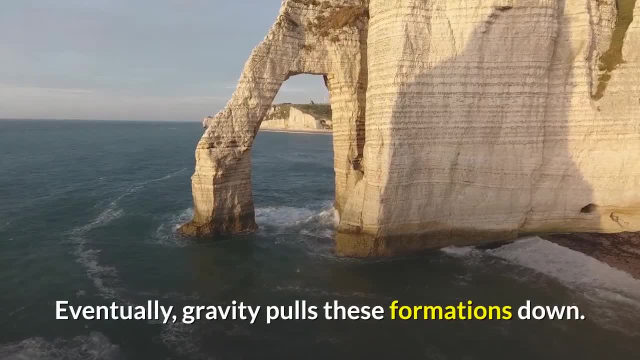 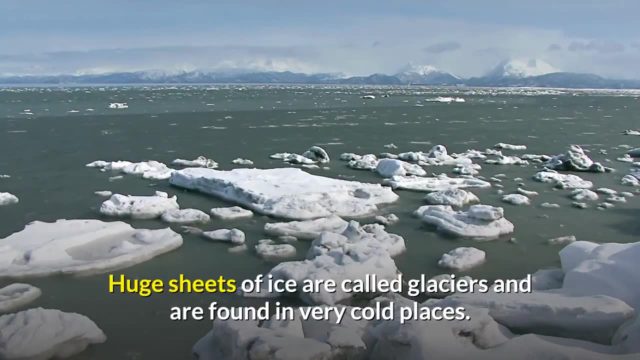 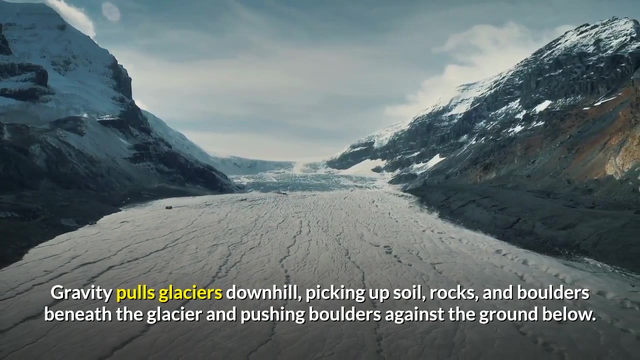 formed by water but shaped by the wind. Eventually, gravity pulls these formations down. Huge sheets of ice are called glaciers and are found in very cold places. Gravity pulls glaciers downhill, picking up soil, rocks and boulders beneath the glacier and pushing boulders against the ground below. 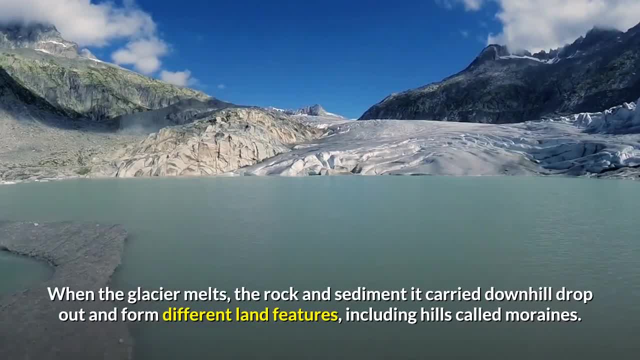 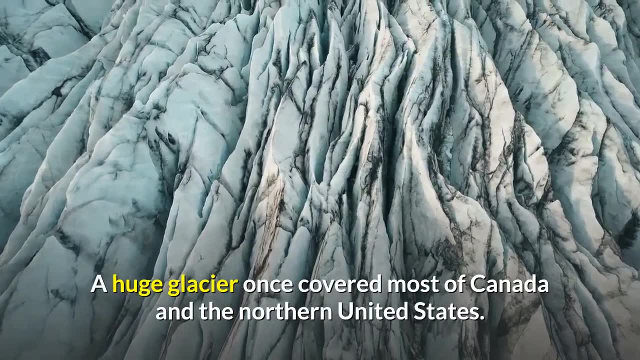 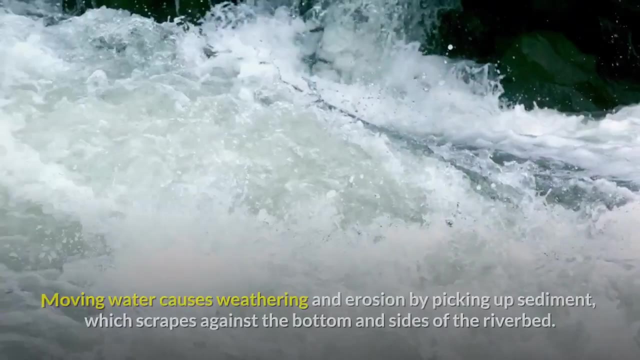 When the glacier melts, the rock and sediment it carried downhill drop out and form different land features, including hills called moraines, A huge glacier once covered most of Canada and the northern United States. The ice cut deep grooves that formed the Great Lakes. 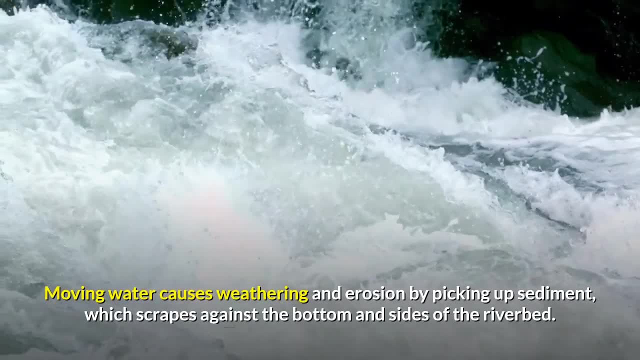 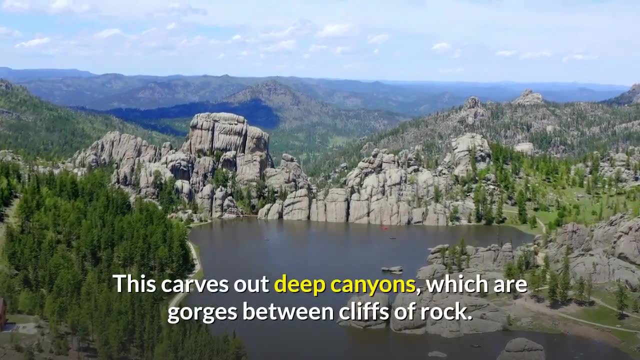 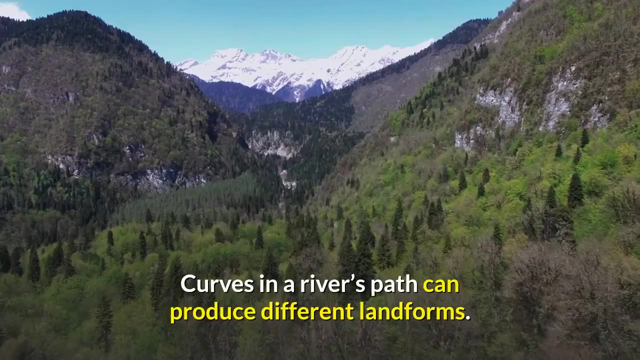 Moving water causes weathering and erosion by picking up sediment which scrapes against the bottom and sides of the riverbed. This carves out deep canyons which are gorges between cliffs of rock. Deposits of sediment can change the direction of river. water Curves in a river's path. 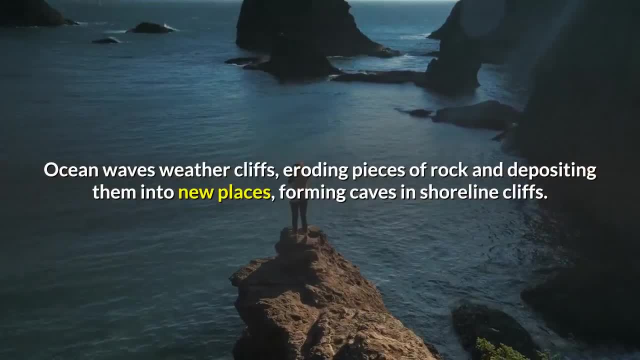 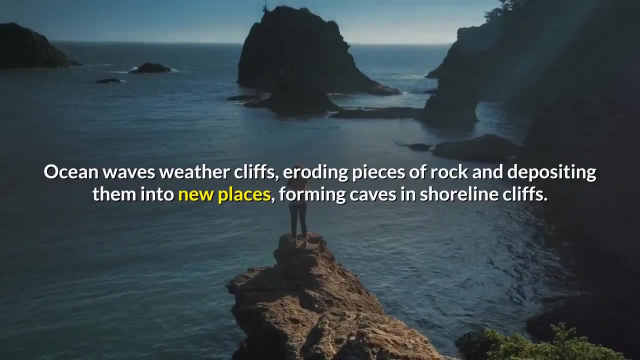 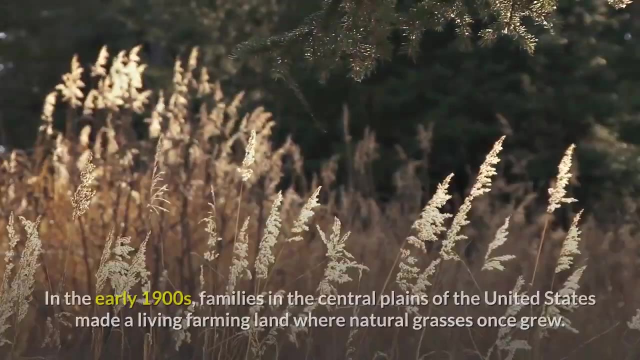 can produce different landforms In waves, weather, cliffs, eroding pieces of rock and depositing them into new places, forming caves in shoreline cliffs. The sediment from eroding shorelines becomes fine sand and beaches are formed at the water's edge. 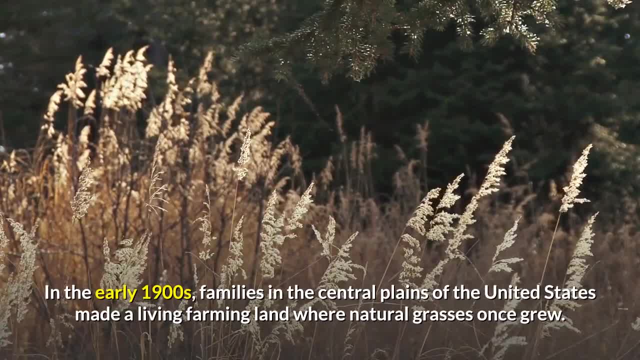 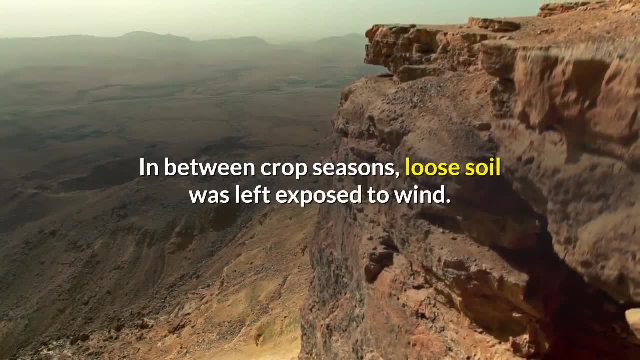 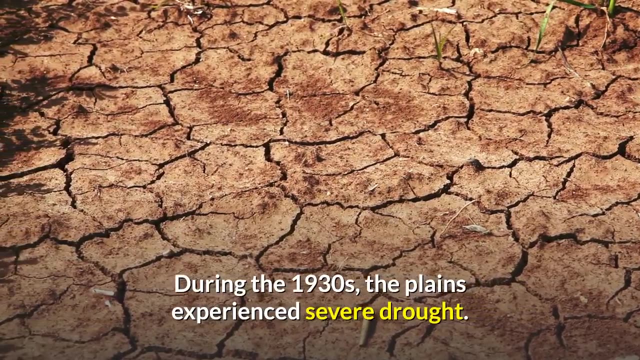 In the early 1900s, families in the central plains of the United States made a living farming land where natural grasses once grew In. between crop seasons, loose soil was left exposed to wind. During the 1930s, the plains experienced severe drought, The soil turned to fine dry dust and high winds. 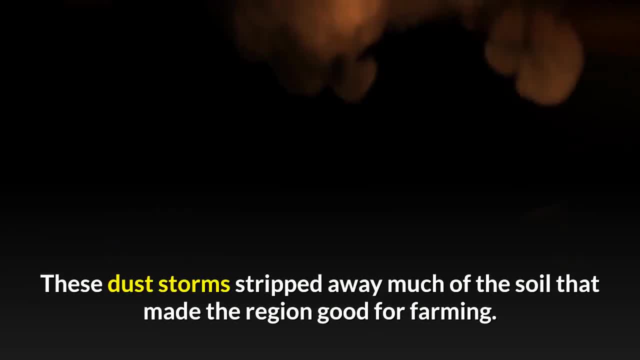 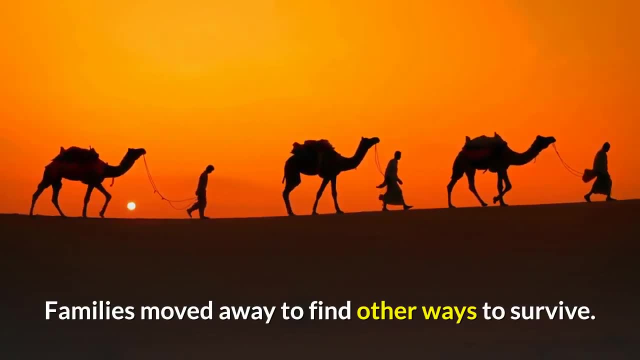 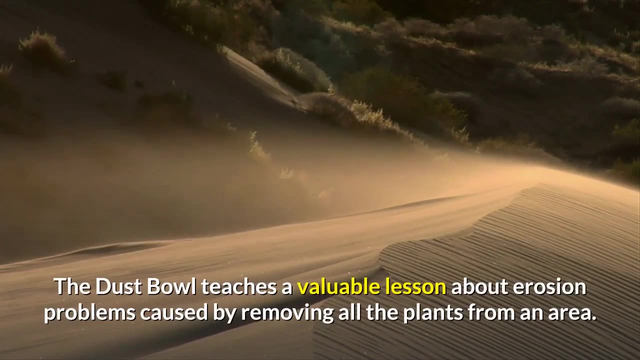 caused giant dust storms. These dust storms stripped away much of the soil that made the region good for farming. Families moved away to find other ways to survive. They suffered hard times. The region became known as the Dust Bowl. The Dust Bowl teaches a valuable lesson about erosion problems caused by removing all the 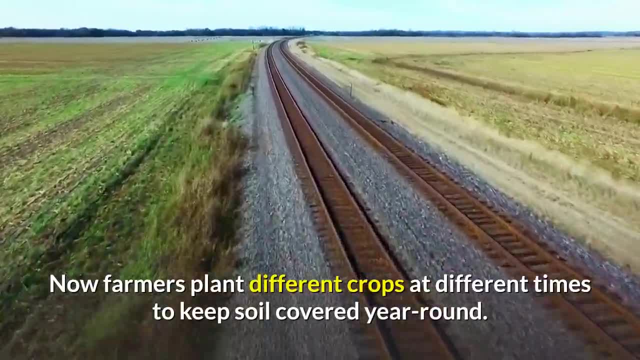 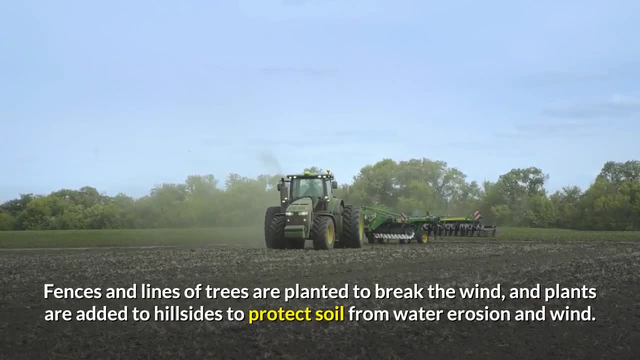 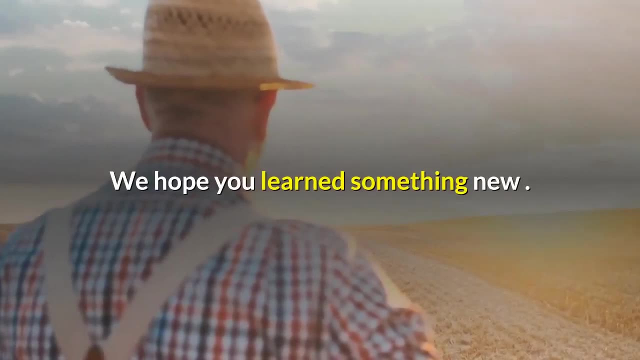 plants from an area. Now, farmers plant different crops at different times to keep soil covered year round. Fences and lines of trees are planted to break the wind, and plants are added to hillsides to protect soil from water erosion and wind. We hope you learned something new. Don't forget to subscribe to receive every new video.